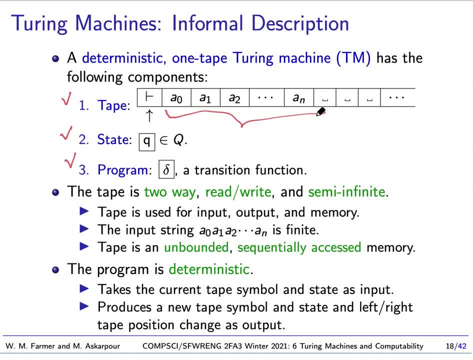 the process of processing of the machine. It will hold a finite string that will then be followed by an infinite set of blank symbols. So the tape we can think of as unbounded, sequentially accessed memory. So unbounded means we can have as much memory as we want and it's sequentially accessed. 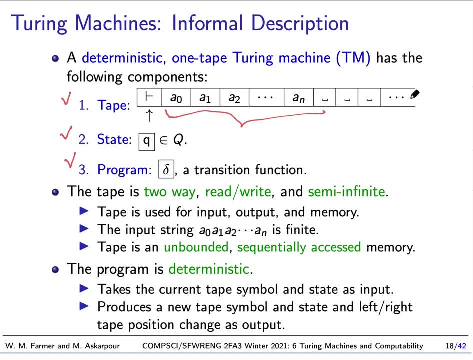 means we get to any point by moving steps to the right or steps to the left. Now the program is deterministic. That means if we have a current state symbol- like we're looking at this symbol- and we have a particular state, the transition function will move us left or right, It will. 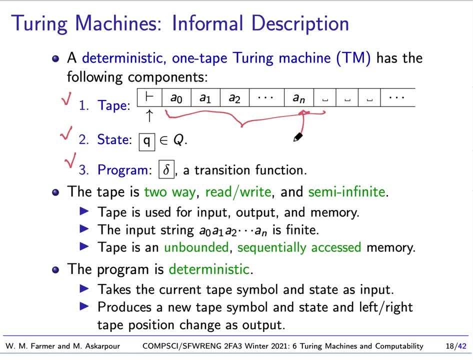 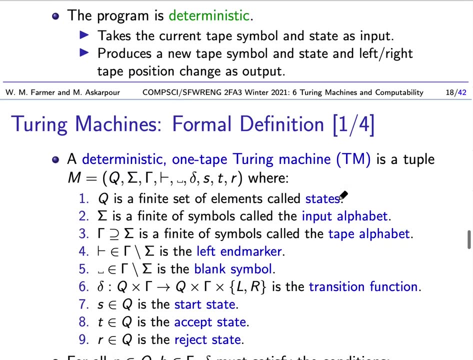 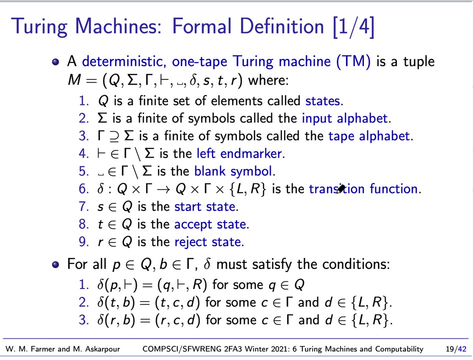 change, possibly the symbol, And that's it. That's all it will do and we'll move to a new state. Now here's the formal definition, And this is a definition for a deterministic one-tape Turing machine. And there's many kinds of Turing machines. Some are indeterministic, Some have multiple tapes. 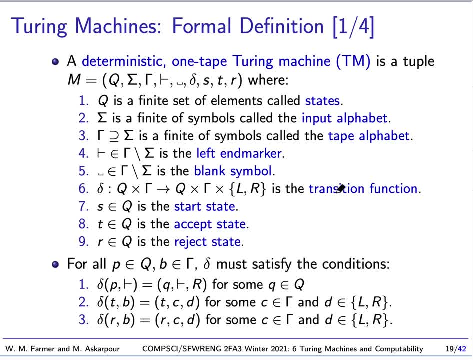 But for us we're going to use the definition of a Turing machine That's deterministic, It has one tape- and this definition follows Kozin's book- And, like our other machines, it's presented as a tuple. So we have Q, which is a finite set of states. We have sigma, which is our input alphabet. 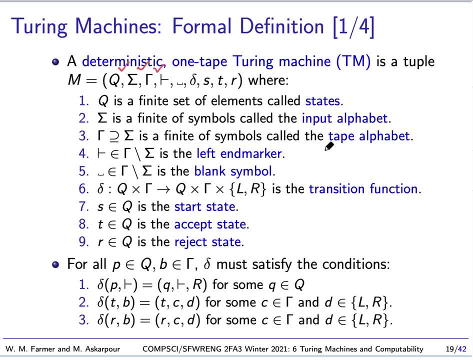 gamma, which is our tape alphabet, which includes all the members of sigma, and then we have a left end marker. that's going to be a symbol, which is in our tape alphabet but it's not a member of sigma, and we have some kind of blank symbol. we have our transition function, which is right here. 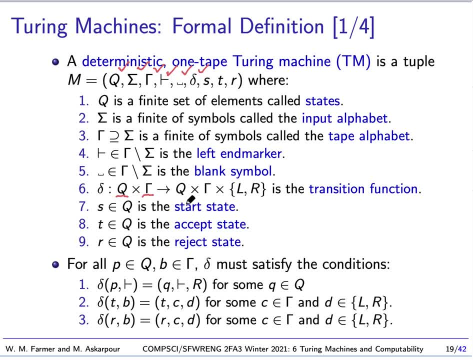 it takes a state, it takes a member on the tape and it produces a new state, possibly overwrites the member that was on the tape, and then it moves either left. the tape head moves left or right and then we have a start state, the state we start in, and a accept state and a reject state. 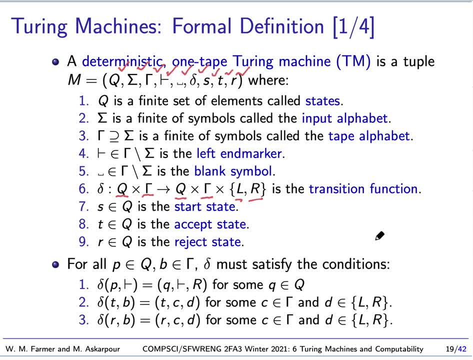 and delta can be almost anything delta- we're very free what delta can be. the only requirements are: if we're in some state and we're looking at the left end marker, we must not overwrite the left end marker and we must move right. so whenever we get to the left end marker, we have to leave it there. 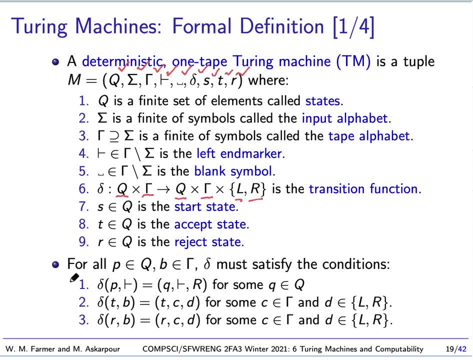 and then move right and the other. so that's one condition. the other condition says that once we're in the accept state, we say we stay in the accept state, we can't ever get out of it and what the machine does doesn't matter, it just keeps running, we stay in that state. 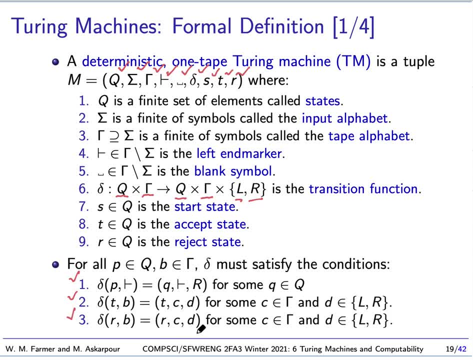 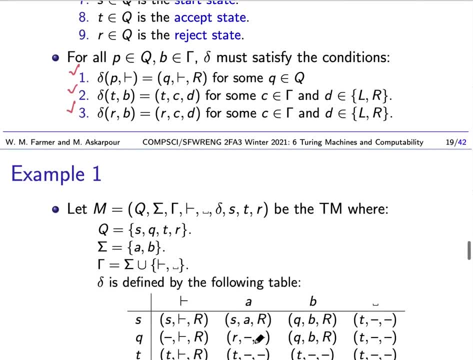 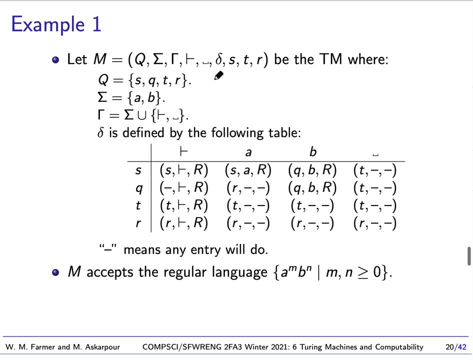 if we end up in the reject state, we stay in the reject state, and what we do when we're in the reject state doesn't matter, okay, so let's look at an example. i'll tell you ahead of time that this example is an example of a 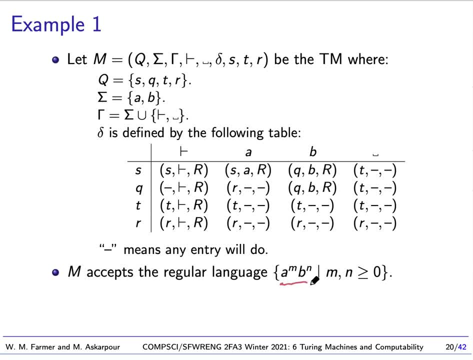 machine and it's going to accept this language: a to the m, b, the n, when m and n are natural numbers. and so we have four states: s, q, t and r- and our input alphabet has two symbols, a and b, and our output alphabet has the symbols a and b, plus the left end marker, plus. 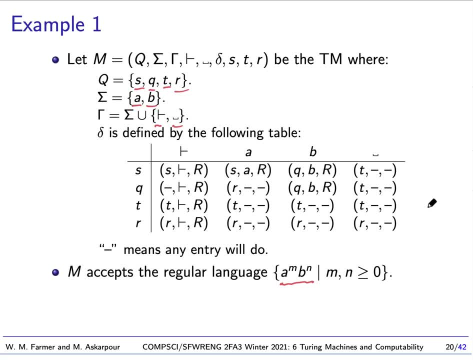 and so this table tells us exactly what delta does. the first thing to notice is that remember when we're reading. so if we're in one of these states and we're reading the left end marker, then we have to. we can change a state to whatever we want, but we must preserve this marker, that's. 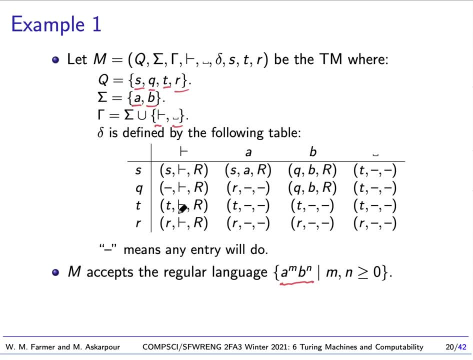 what this means and we go right. so this is 1 X 0 and we're going to do: now: this is 90 and we're going. this means and we go right. And so if we're in the start state, we're going to stay in the start. 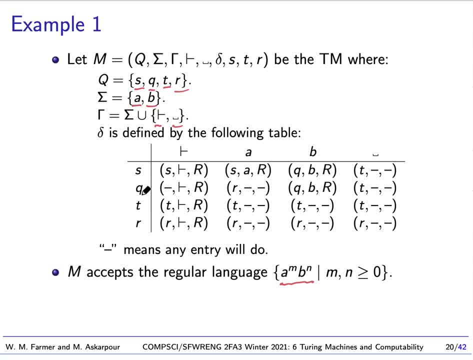 state. If we're in the state Q, it doesn't matter where we go, because we're never going to get in this situation where we're in state Q, looking at the left-hand marker, And of course, if we're in the accept state or reject state, we stay in those states And notice we put these dashes. 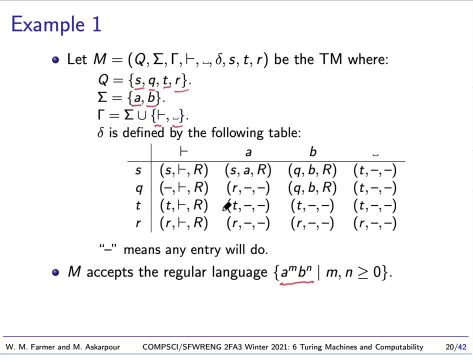 meaning it doesn't matter what we put here, We can put whatever we want. So the important things about the accept state and reject states: once we're in them, we stay in them, And so basically, the real key of what's happening is in states S and Q, And so state S, what it does is we're 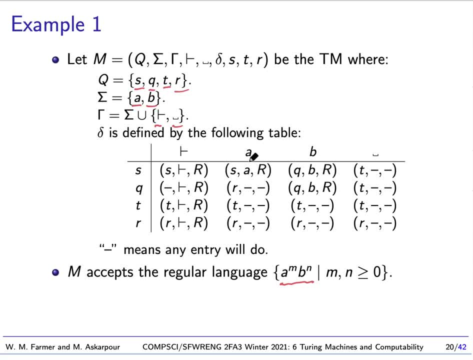 looking for an A, And so if we're in state S and we see an A, we go to the right and we stay in S. If we end up seeing a B, then we go to state Q And in state Q, if we see any A's we reject. 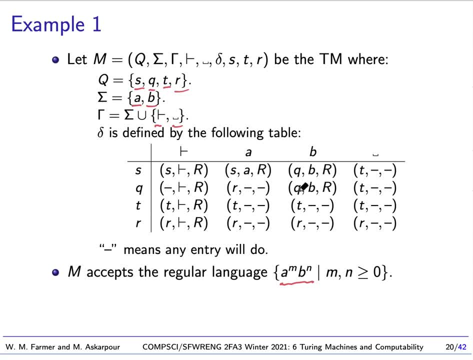 If we see a, Q- excuse me, if we're in Q and we see a, B, then we move to the right, And if in either state we see a blank, then we accept. So basically, think of it this way: We're going to start with. let's see, we're starting with. 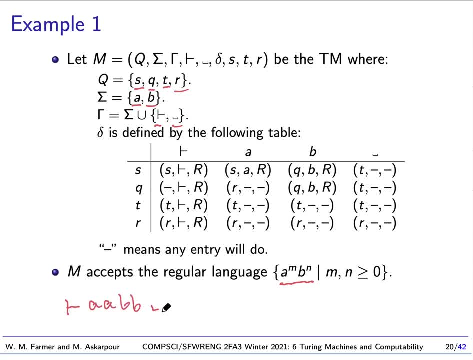 A, A, B, B, and then we have a bunch of blanks here. So we start here in state S, And then in state S we're reading this: We're going to keep this thing the same And we move to the right. So we're here in state S And then we read an A. We keep the A there. 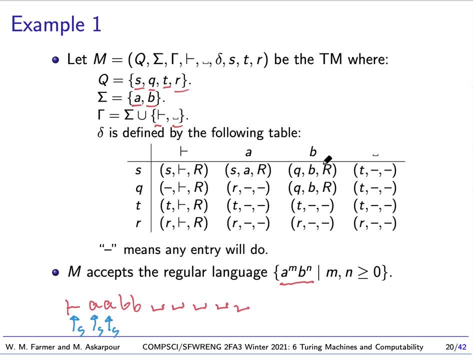 We move this way And then we get, we read this A, And then we move here again to the right, But now we're still in state S, And now in state S we're reading a, B, And now we go to Q. 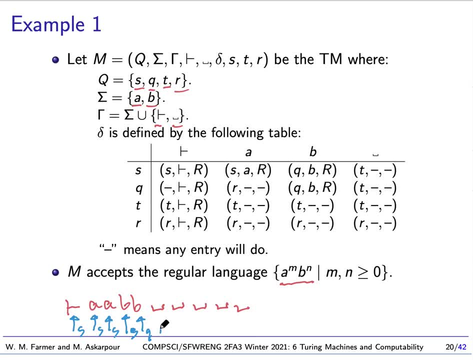 And in Q we're reading a, B, We go to the right And we're in. we go to the right And now we're in state Q. And now we have a blank. And in state Q, what do we do? 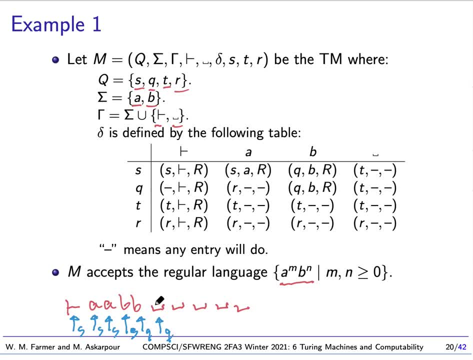 We go to the accept state. So we accepted this Now for B. now we're in state Q, So we accept this. So we accept this Now for B. now we're in state Q. if we had something different, let me use a different color. if we had, let's say, an. 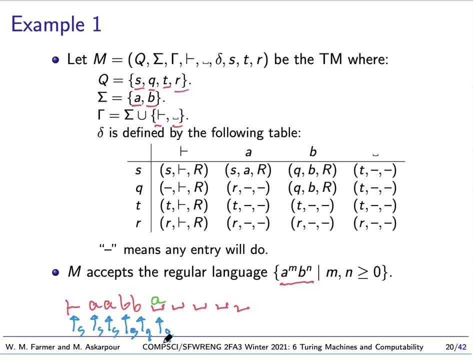 A here, what we'd be happy when we got here in state Q and we're reading an A. then we would go to the reject state. Okay, so that's example one. This is very simple, and notice that we're using a Turing machine, which is a very powerful machine, to simulate a finite. 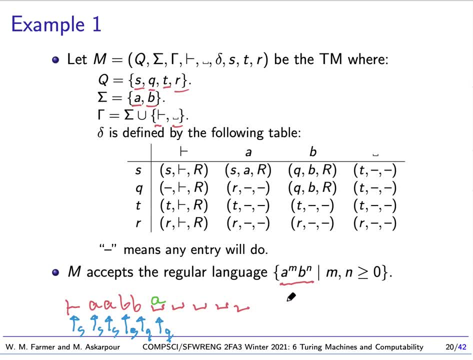 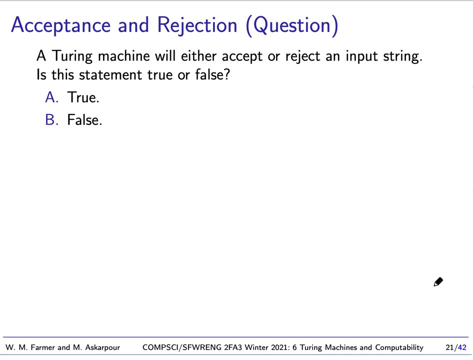 automata because, as you know, this language, this language here, is regular. Okay, so I have a question. A Turing machine will either accept or reject an input string. Is this statement true or false? I'll give you a moment to think about it and come up with an answer. 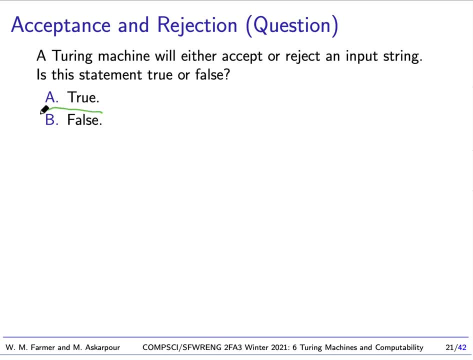 Okay, well, welcome back. The answer is false, Because a Turing machine, if you give it an input, there's three possibilities: It can accept, it can reject. and it can reject loop Looping means it just runs forever. This is different from the other kinds of 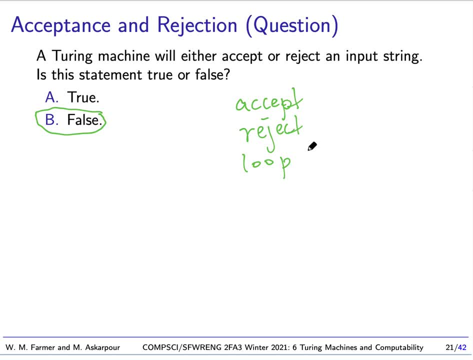 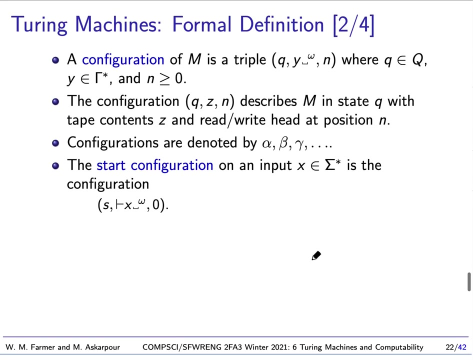 automata that we've seen The other kinds like finite automata and push-down automata. they either accept or reject. But Turing machines have a third possibility: They can loop. Okay, So let's think of what a configuration is. A configuration is going to be a triple. 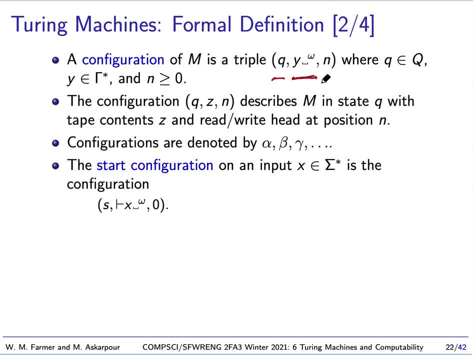 It's the state we're in. It's what's ever on the tape. And what's ever on the tape will be a finite string of tape symbols, followed by an infinite string of blank symbols. Now Y could also include blank symbols, But eventually. 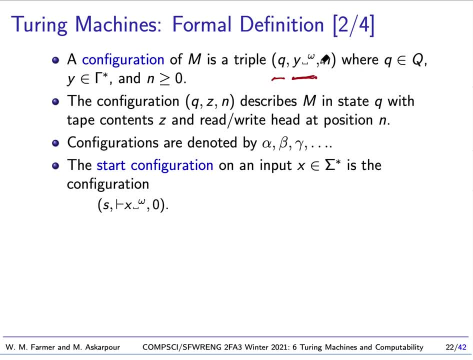 Y could also include blank symbols, But eventually- But eventually- we're going to have an infinite string of blank symbols. now, the this thing that looks like a w is really omega, and omega is the first infinite art ordinal, so we're using omega here to represent. 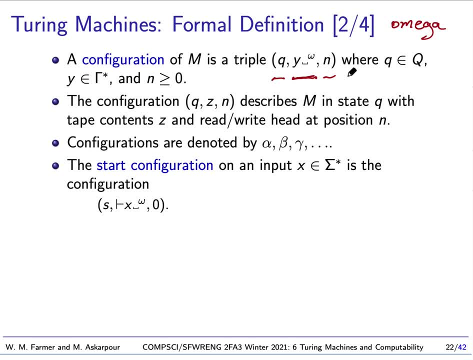 infinity and then finally we have n is where the tape head is where the. so if we have our tape like this at some point, so if we index these like this, the tape head is pointing at that point, and so a configuration describes our machine in state q, with tape content z and the rewrite 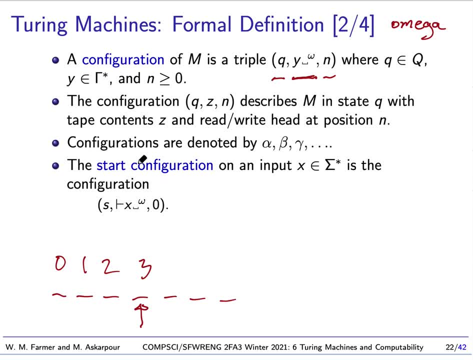 head is at position n and configurations are denoted by greek letters, and the start configuration looks like this: we're in the start state, whatever that is for our turning machine, we have always the left end marker, we have our input string and then we have an infinite string of blank symbols and we're 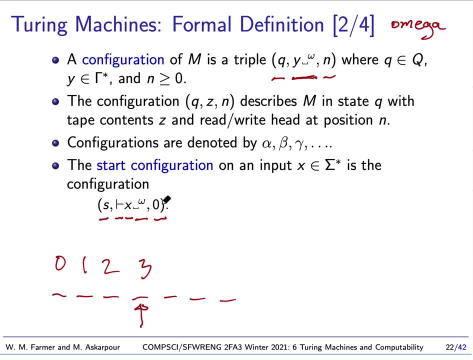 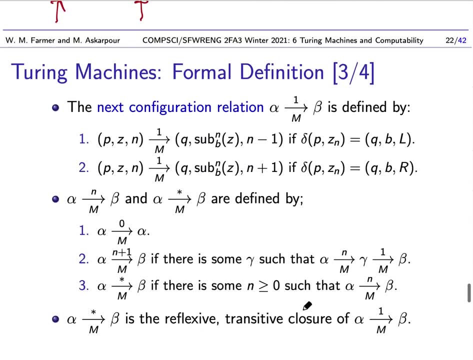 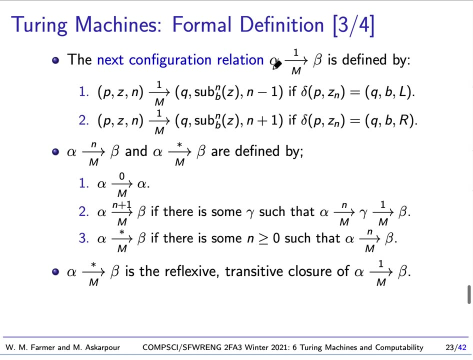 we're, uh, the tape head is pointing to the first position that will be right here, which will always be the left end marker. okay, so then we can define our next configuration relation, how we get from one configuration to the next. it's, it's pretty simple: if we're in state p and we're in state p and we're uh looking at a string z, 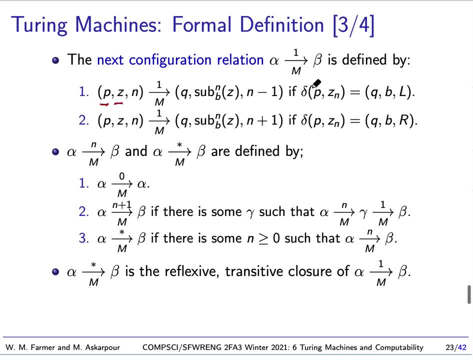 and there is a transition that says for p and the symbol, the symbol at the nth position in Z. If we have a transition for that, well we will. I'll have a transition for every possibility here, But the symbol at the nth position in Z. we'll use that transition to. 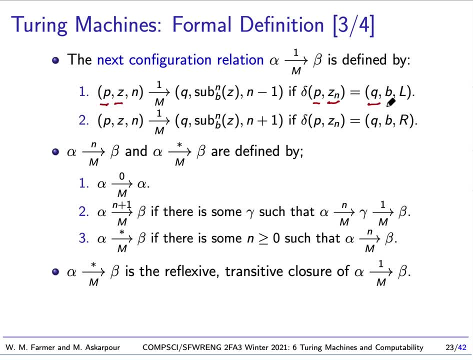 go to a new state. We will rewrite the symbols at the nth position with B and we will move to the left. So that's what this says. We'll go to the new state Q. We will substitute into our string. We will basically replace: at the nth position. We will replace whatever. 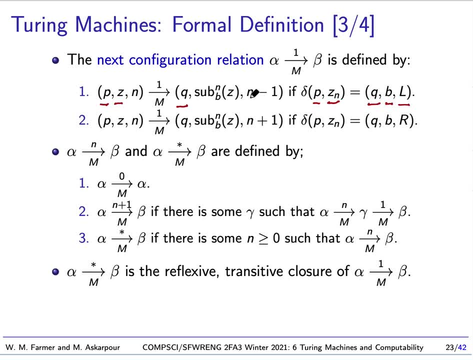 is there by B, and then we will move the tape head backwards to the left one, And if we have right, everything's the same, except we move forward. And then we can define these relations just as you've seen before. And there's nothing really new there. 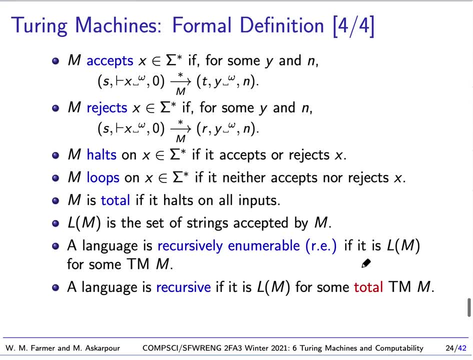 Okay, So we need to introduce some more definitions. Our machine accepts a string if we start off with that string on the tape X. So we're trying to accept X, It's on the string And we eventually get to a accept state. 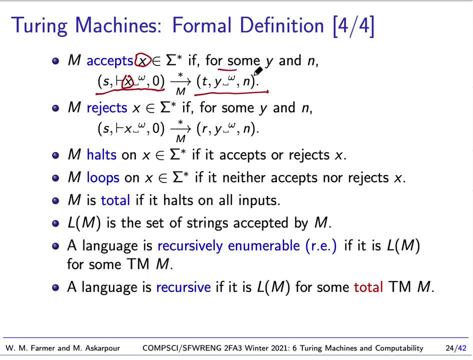 The accept state And it doesn't matter what's here and here, It doesn't matter this part. What matters is that we get to the accept state And we reject. if we start the same way but we end up in the reject state And it halts if it either accepts or rejects and it loops if. 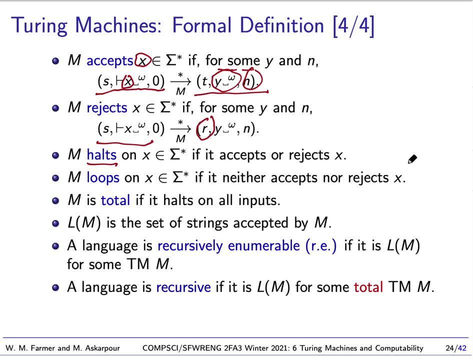 it neither accepts nor rejects And loops, let me repeat, is just what it sounds like. The machine would just keep going from state to state, moving around the tape, doing a lot of things, but it will never stop. And we say M is total if it halts in all inputs. And the language of M is a set of strings. 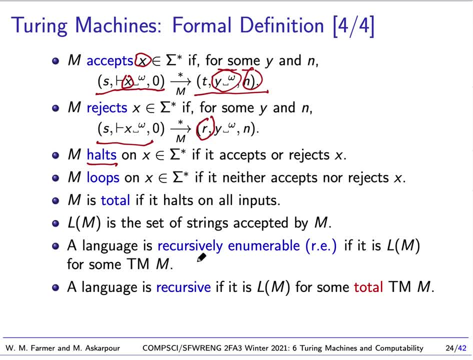 accepted by M And a language is called recursively enumerable if the language is accepted by some Turing machine And it's recursive if it's accepted by some total Turing machine. So if we think of all the RE languages like this recursively enumerable language, it contains the set of recursive languages And these are sitting in the big 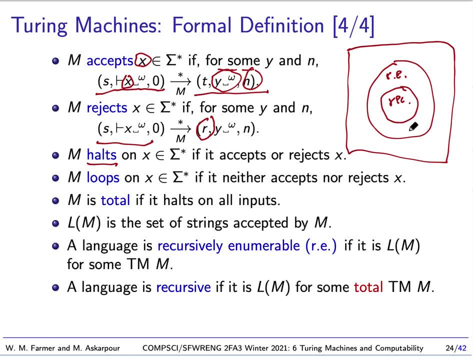 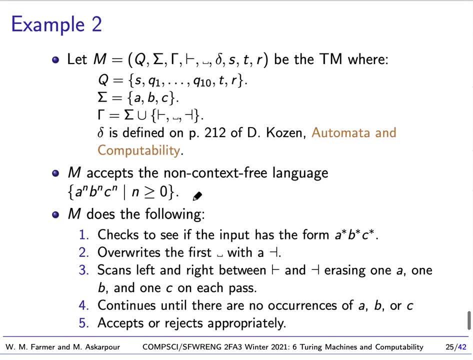 space of all possible languages. Okay, So let's look at one more example. This is an example of a set of recursive languages. For example, for a non-context-free language, it's A to the n, B to the n, C to the n. when 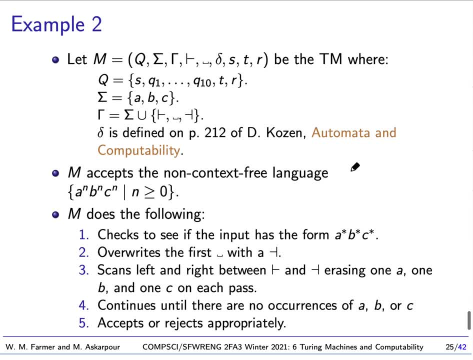 n is greater than or equal to 0.. And we know that this is non-context-free because we have talked about how you can use the pumping lemma for context-free languages to show that this is non-context-free. It is accepted by a Turing machine. It's accepted by this Turing machine M. Therefore, this: 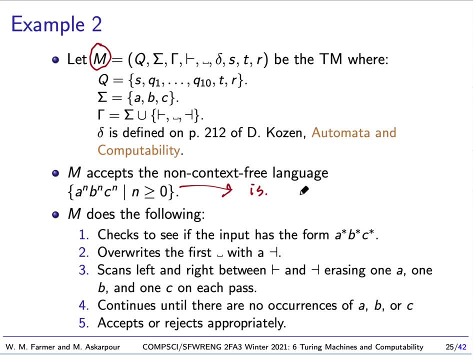 language is recursively enumerable, Because all languages accepted by Turing machines are recursively enumerable, And this is defined on page 212 in Kozen's book. We have a start state, then 10 other states and we have the accept state and reject state. We have just these three input symbols. 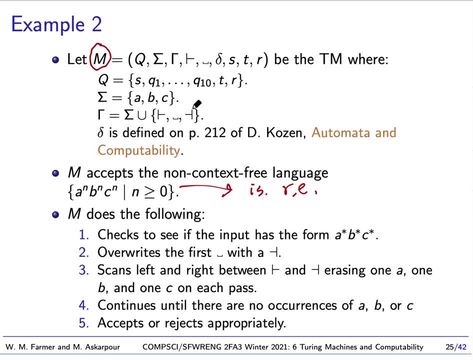 and we have an extra tape symbol: the write and marker. So how does this work? Well, the way this works is it first. so we're going to start off with some string And we're hoping the string looks like this. And so the first thing, 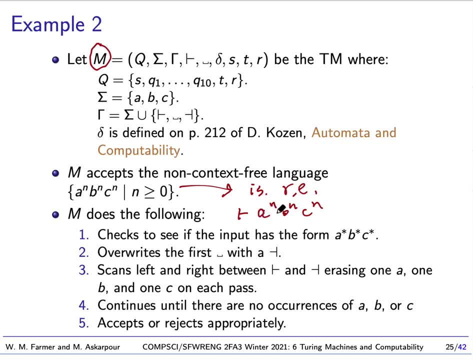 we do is our machine keeps reading A's And when it gets done it reads B's, and then, when it gets done, it reads C's, And if it finds any, you know, after reading A's it finds some B's and A's it's going to reject. 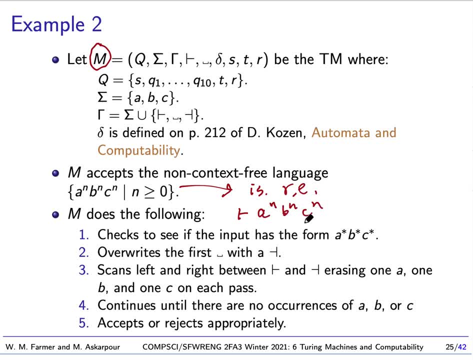 But if it reads that there's just A's and followed by B's and followed by C's, it will put this marker at the end And then. so that's what it would do, number 2. Then it would go back and forth And each. 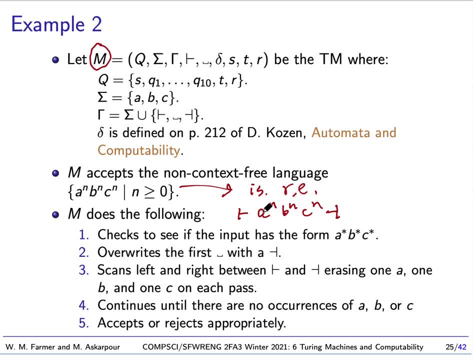 it goes back, it will start with an A and it will replace an A it finds with the blank symbol. Then it will look for a B and replace it with a blank symbol. Then it will look for a C and replace it with a blank symbol. Then it will go back to the left again and